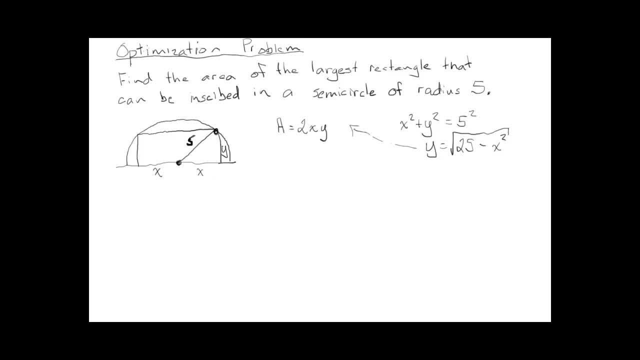 Now I'm going to show you a different way to do that, to do this question, and this is using trigonometry. So what I'm going to do is this right angle triangle. I'm going to let theta be this angle here. 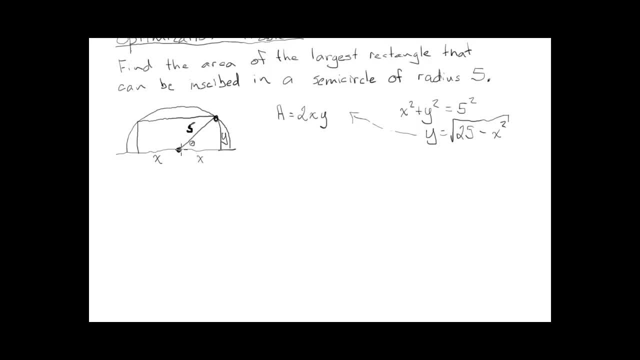 Um, and then I have my basic trig ratios. so the cosine of theta is equal to the adjacent side, which is X over 5.. The sine of theta would be equal to the opposite side, which is Y over 5.. So X is. 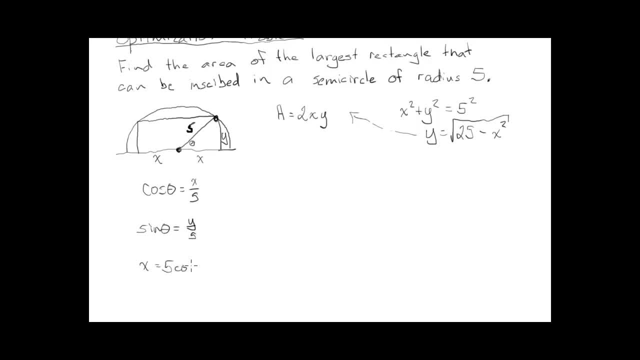 O' O'. So X is is equal to 5 cos theta, and y is equal to 5 sin theta. So now what I'm going to do is I'm going to take both these things and sub them into this equation up here. So the area. 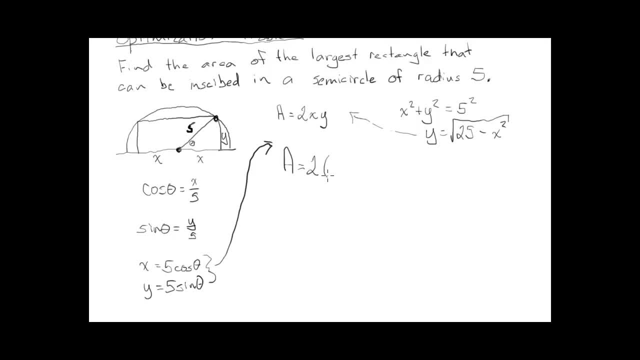 equals 2 times 5 times the Cos theta times 5 times the sin theta. Putting that all together you get well, the 5 times a 5 is 25.. I'm going to move the 2 to, So I'm not going to expand 25.. 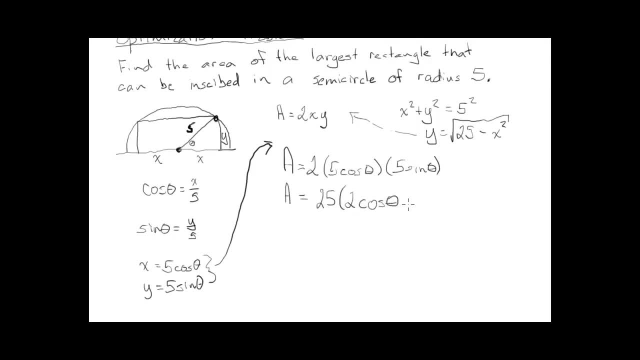 So I'm not going to expand 25.. 25 times 2, and the reason is that's going to let me simplify this a little bit. Notice this thing: right here inside the bracket, that's your double angle formula for sine 2 theta right: sine 2 theta equals 2 sine theta cos theta. so I'm going to make that. 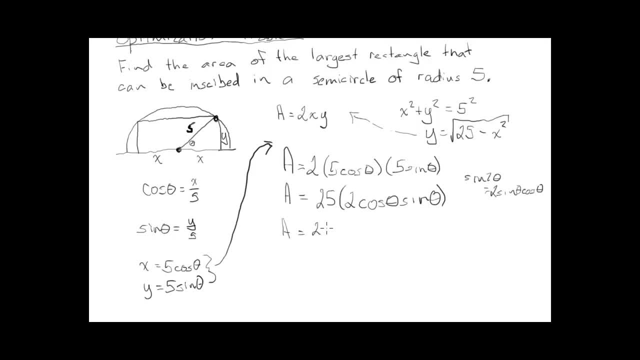 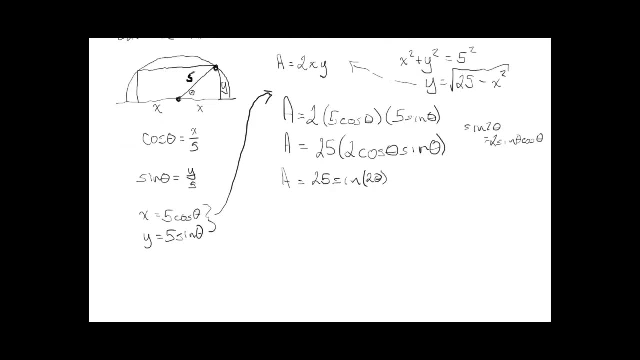 substitution. now the area is equal to 25 times sine of 2 theta. and now I have a function for area in terms of just one variable. that variable is theta, so I should be able to take the derivative, set it equal to 0, and find the critical numbers. 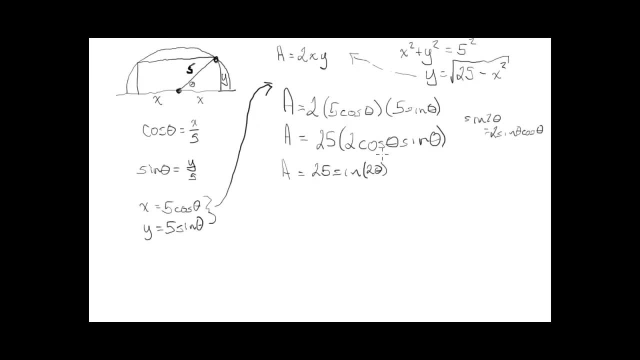 I could have done this without making the substitution and having cos theta sine theta, but then I would have to use the product rule. so it's just a little easier if you recognize this identity. so I'm going to differentiate with respect to theta. so 25, I'm going to 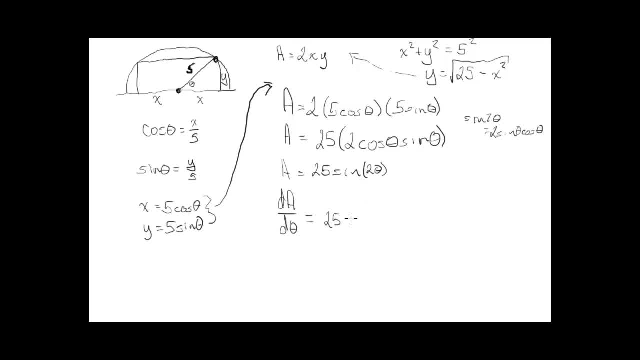 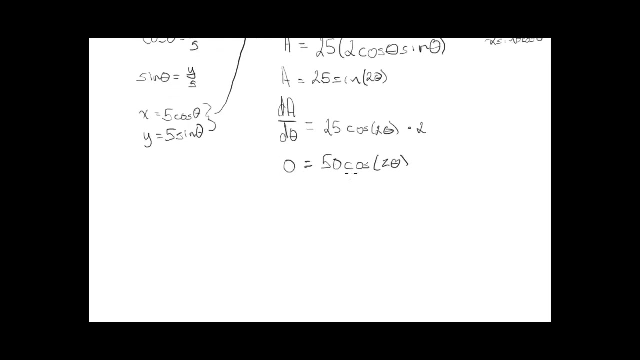 get 25,. the derivative of sine theta is cos theta, cos 2 theta times the derivative of 2 theta, which is 2, so setting the derivative equal to 0, I'll get 50 cos theta and then 2 theta. so when does cos 2 theta equal 0?? 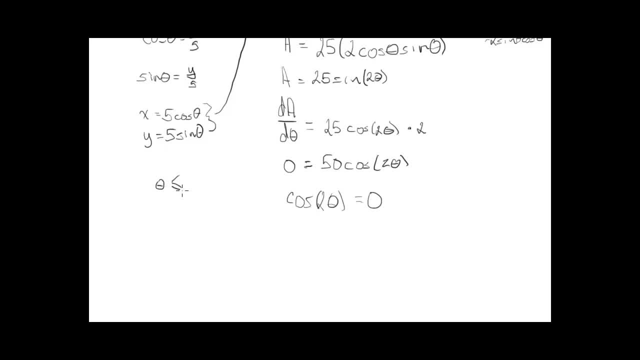 Remembering that theta was an angle in a right angle triangle. so it must be less than pi by 2, but bigger than 0, which means 2 theta must be less than pi but bigger than 0, so when does 2 theta equal 0?? 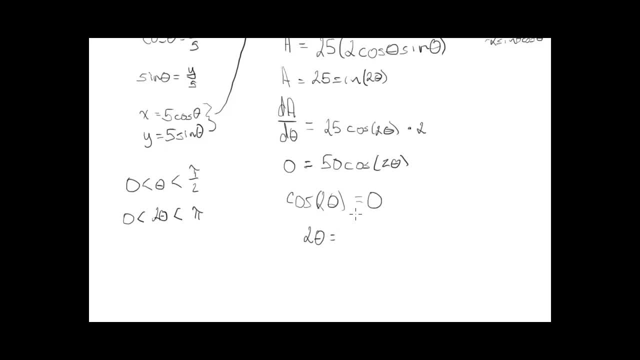 The derivative of sine is 0 at pi by 2, dividing both sides by 2, I get pi by 4, so this is the critical number. Now I just want to show that This was a maximum. so remember theta was between 0 and pi by 2 was the critical number. 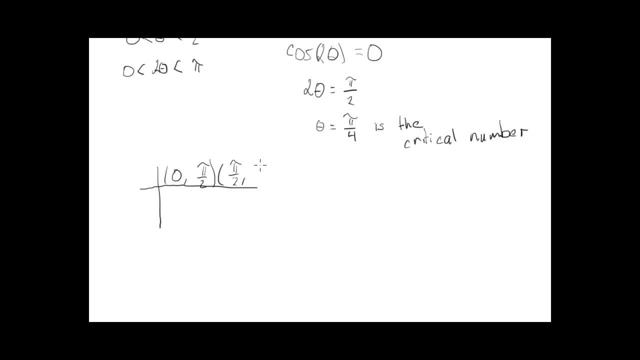 so pi by 2 to pi by 4, pi by 4 was the critical number and then pi by 2.. So I have to look at dA or d theta by d Sorry, dA by d theta. So remember, dA by d theta was. 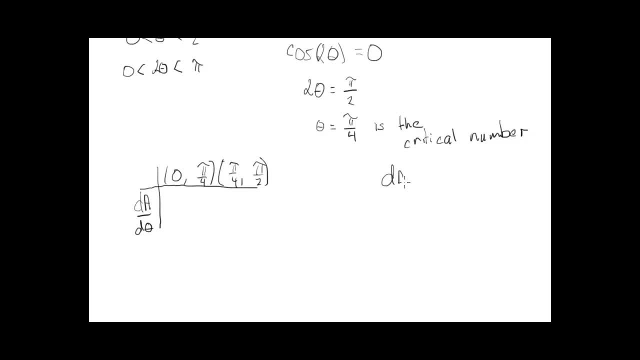 Just remind us, dA by d theta was- I think it was- 50. Cosine 2 theta. So if you took a number between 0 and pi by 2, cosine would- dA by d theta would be positive.